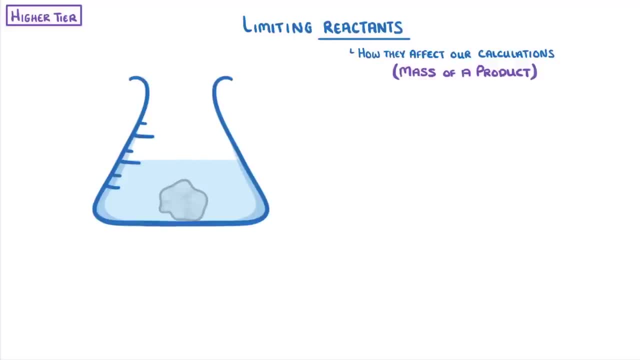 acid and we dropped in some calcium carbonate. As the hydrochloric acid and calcium carbonate react, they'll produce calcium chloride, water and carbon dioxide And we'll be able to see that a reaction is taking place because the solid calcium carbonate will slowly disappear. 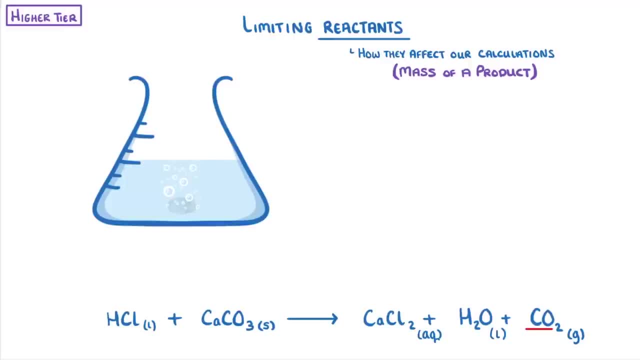 and bubbles of gas will be given off, which is our carbon dioxide. After a while, though, all the calcium carbonate will disappear and the fizzing will slow down and eventually stop. So at this point, we know that one of our reactants must have all been used up. 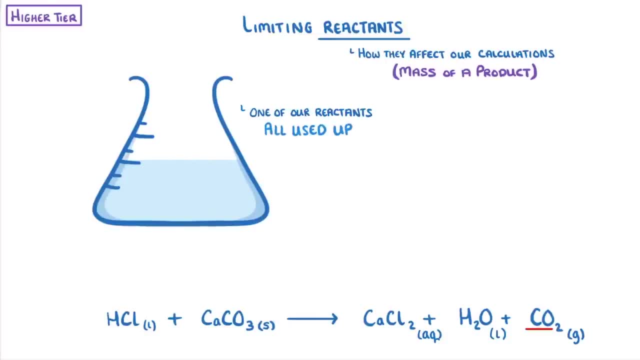 because the reaction stopped. If we can see that the calcium carbonate has all disappeared, then we know that it must have all been used up, and so we would call it the limiting reactant, because it limited how much product could be produced. On the other hand, there's probably still loads. 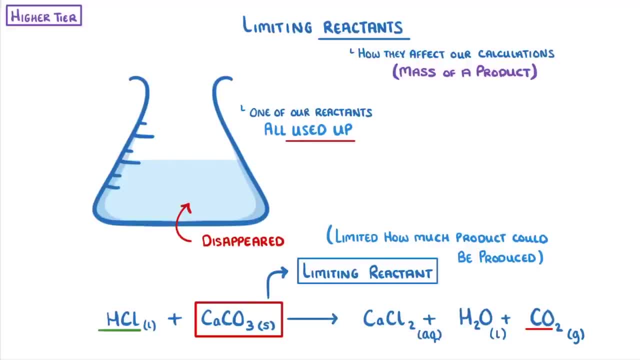 of hydrochloric acid left, so we would say that the hydrochloric acid is in excess. The reason this is important is because how much product we get depends entirely on the limiting reactant. For example, if we add more calcium carbonate, we'll see more fizzing. 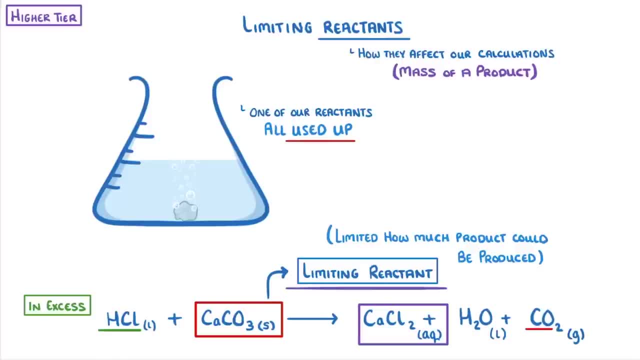 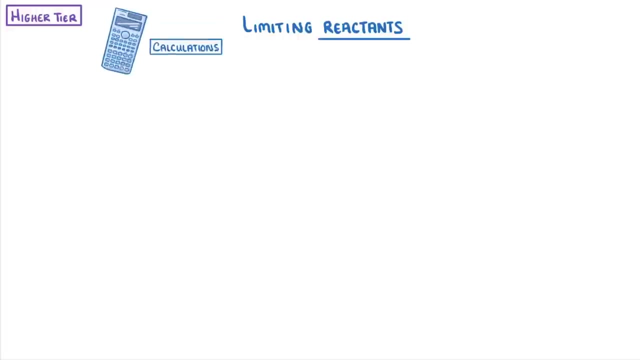 as more products are made, However, this fizzing would stop as the calcium carbonate is used up again, Whereas if we add some more hydrochloric acid, then nothing will happen because it has no calcium carbonate to react with. Now, when it comes to calculations, you will sometimes be told that one of the reactants 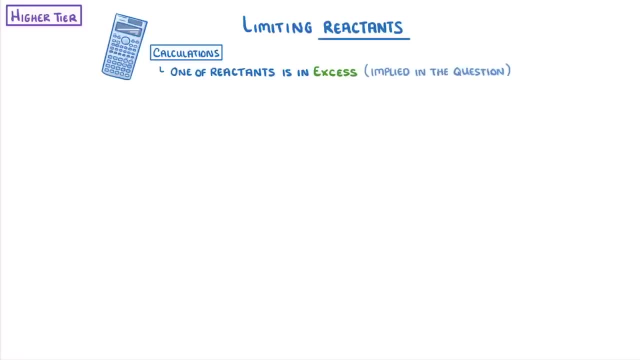 is in excess. In other cases, though, it might just be implied in the question. For example, calculate the mass of sodium oxide produced when 115g of sodium is burned in air. Burning in air is known as combustion and basically just means reacting with oxygen. 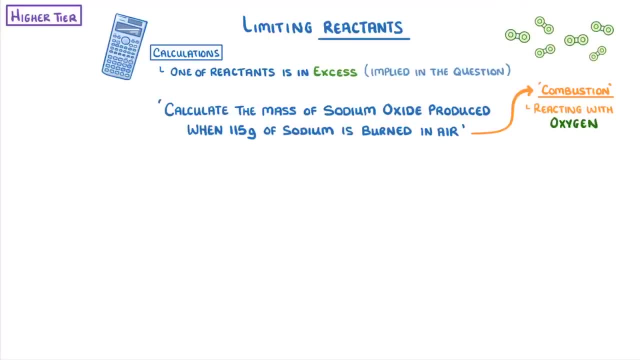 And, if you think about it, there's loads of oxygen floating around in the air, so we can assume that the oxygen will be the one in excess, which means that our sodium must be the limiting reactant. The first step with any question like this is to write out the equation and then balance.